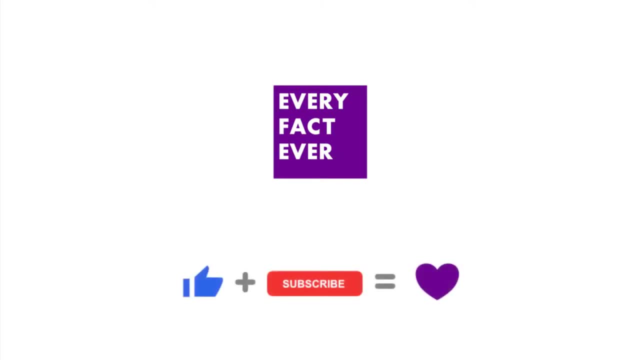 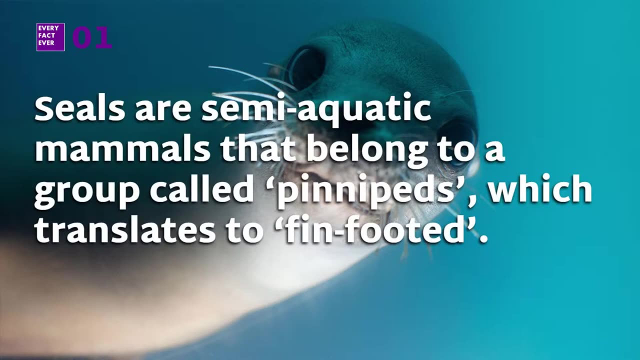 Welcome to Every Fact Ever. Like and subscribe for more amazing facts. This is 50 Facts About Seals. Fact Number 1. Seals are semi-aquatic mammals that belong to a group of pinnipeds, which translates to thin-footed Members of this group, are characterised by having front and rear flippers. 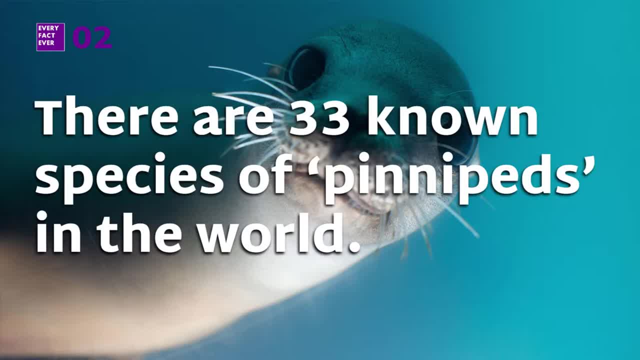 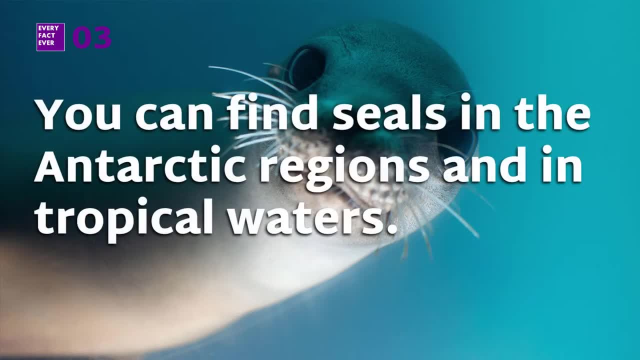 Fact Number 2. There are 33 known species of pinnipeds in the world. Scientists believe that pinnipeds have evolved from terrestrial otter-like creatures. Fact Number 3. You can find seals in the Arctic regions and in tropical waters, When seals are. 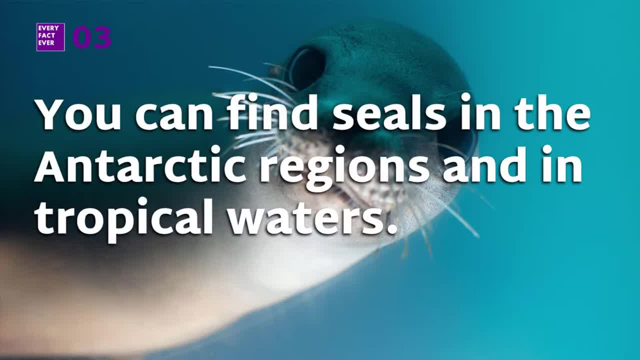 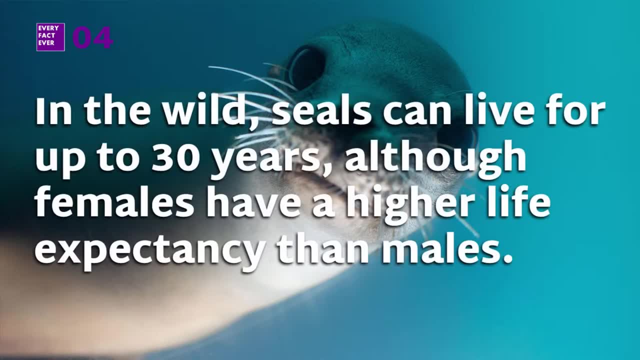 not lazing about under the sun, they unleash their amazing prowess as efficient predators in the Atlantic waters. Fact Number 4. In the wild, seals can live for up to 30 years. although females have a higher life expectancy than males, Female harbour seals have a life expectancy of 30-35%. 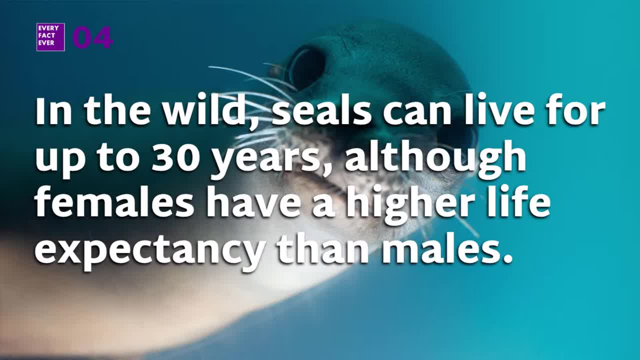 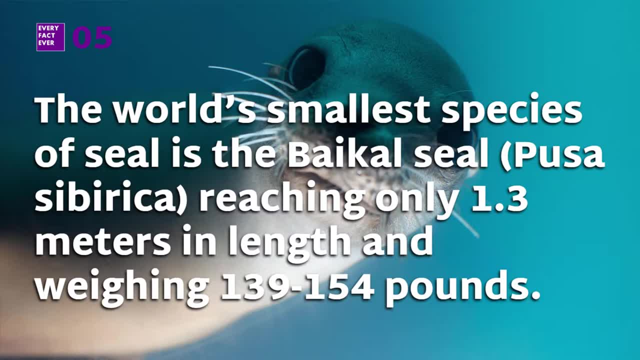 Whereas males only live for 20-25 years. Fact Number 5. The world's smallest species of seal is the Baikal seal, reaching only 1.3 metres in length and weighing 139-154 pounds. This eel seal is anemic to Lake Baltic in Siberia, Russia, and is the only exclusive freshwater pinniped species. 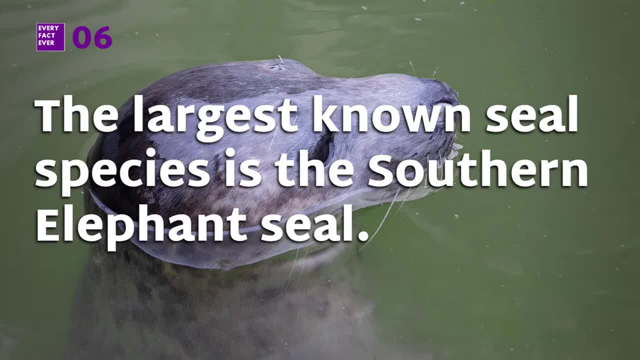 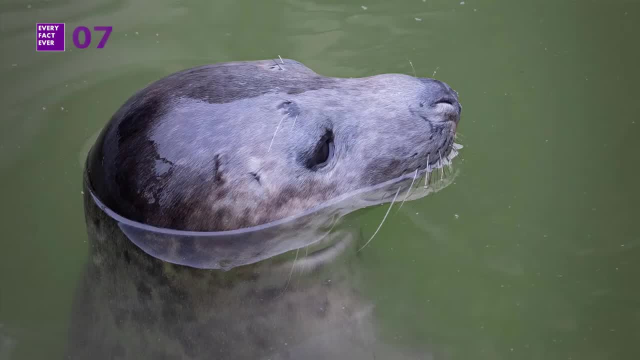 Fact Number 6. The largest known seal species is the Southern Elephant seal. It can reach up to 5.8 metres in length and can weigh up to 8,800 pounds. Fact Number 7. All seals share some general physical characteristics. 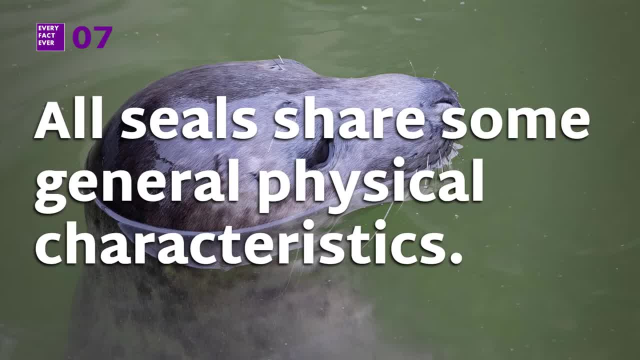 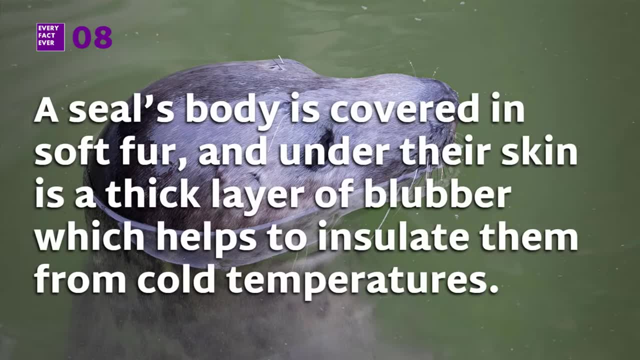 Seals are warm-blooded organisms and have large flippers instead of arms and legs. Fact Number 8. A seal's body is covered in soft fur and under their skin is a thick layer of blubber which helps to insulate them from the cold temperatures. The blubber is a thick layer of fat. 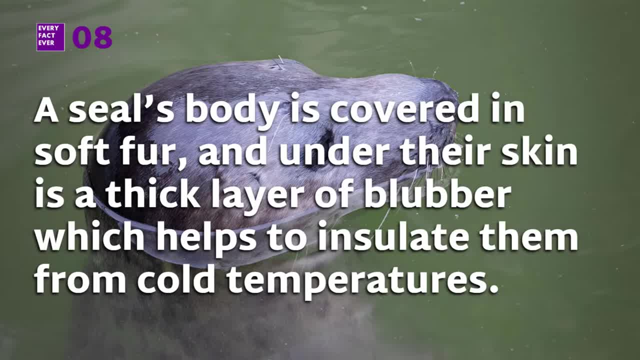 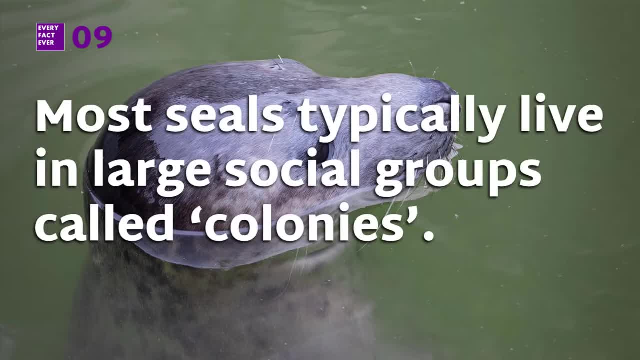 or adipose tissue that stores energy and increases the ability for the seal to breathe. Fact Number 8. The leopard seal is a very aggressive animal and increases the animal's buoyancy. Fact Number 9. Most seals typically live in large social groups called colonies, Each tight knit. 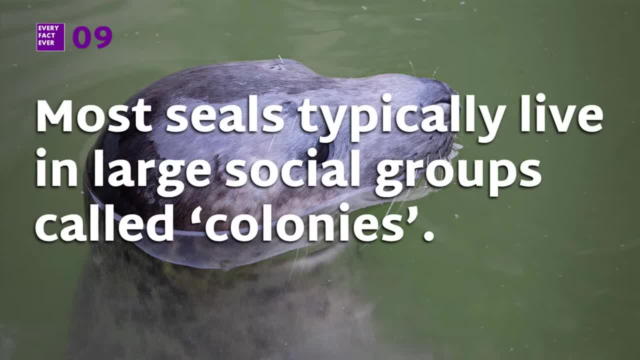 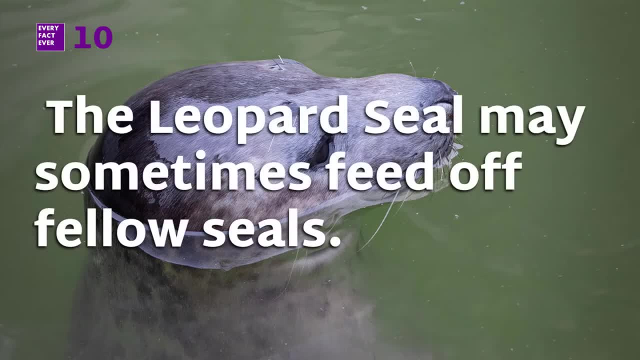 colony can have thousands of members that come together to sunbathe, mate and raise their young. Fact Number 10.. The leopard seal may sometimes feed off fellow seals. They are considered to be the most formidable hunters of all the seal species and are the only ones that prey. 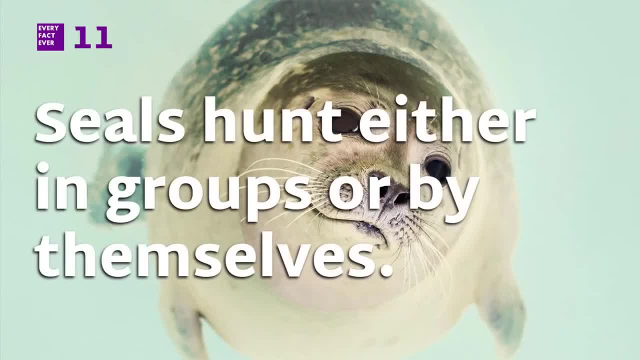 on the warm-blooded animals. Fact Number 11. Seals hunt either in a group or by themselves. Their streamlined bodies enable them to hunt for food in frigid waters with ease. Fact Number 12. Seals have highly sensitive whiskers. 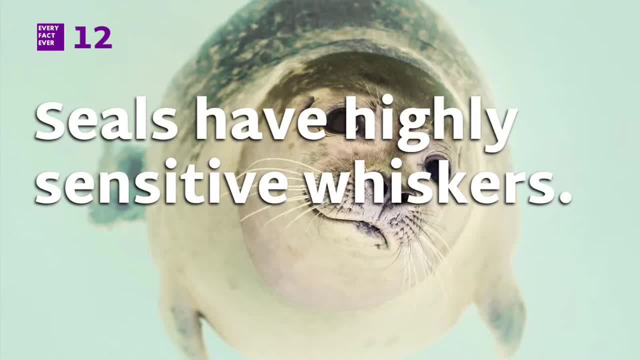 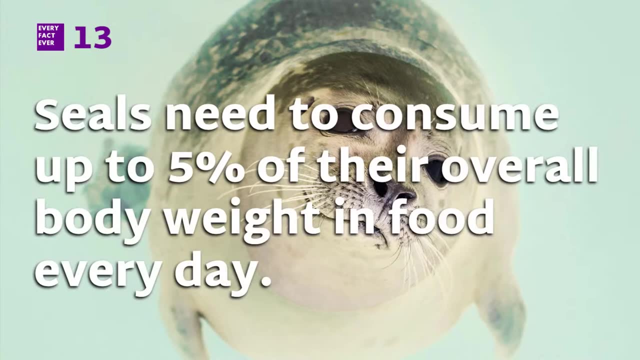 These whiskers can sense movement and vibrations in the water, making seals highly effective hunters. Fact Number 13. Seals need to consume up to 5% of their overall body weight in food every day. It takes them hours to feed each day. 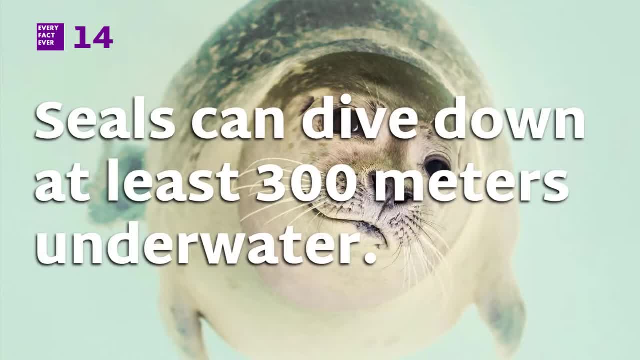 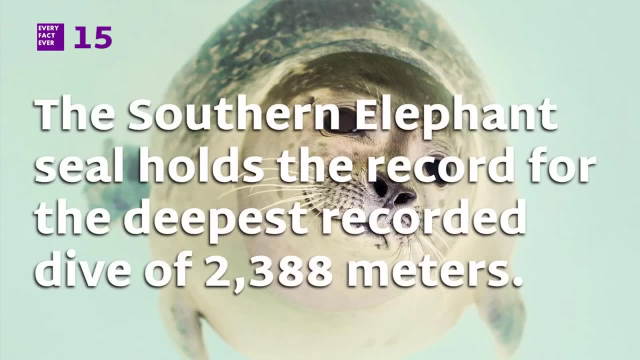 Fact Number 14. Seals can dive down to at least 300 metres underwater. Some species of seal can even dive up to 900 metres when searching for food. Fact Number 15. The southern elephant seal holds the record for the deepest recorded dive of 2,388 metres. 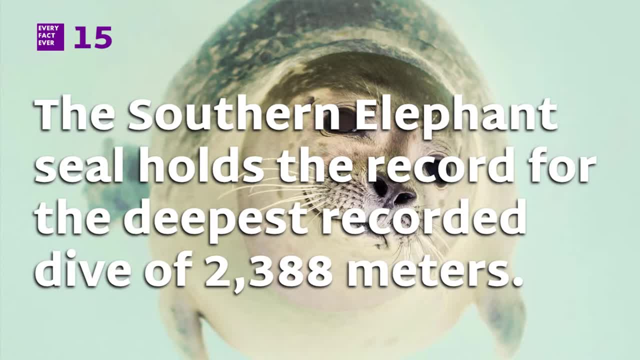 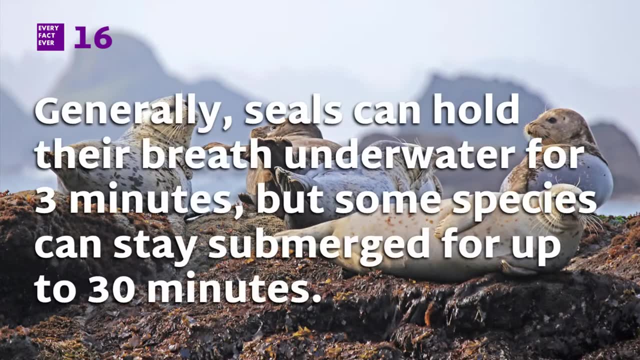 This species' diet consists of deep-dwelling animals such as rays, skates, octopus, large fish and squid, hence the deep diving Fact Number 16.. Generally, seals can hold their breath underwater for 3 minutes, but some of the species can. 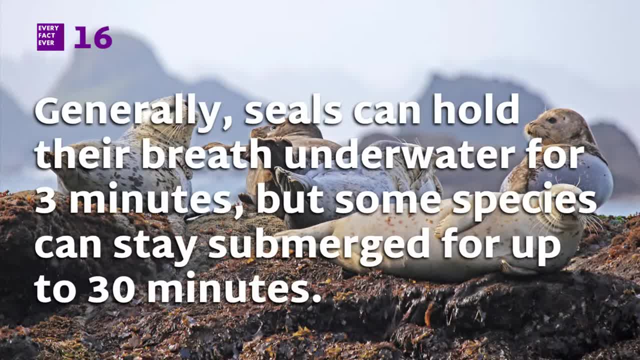 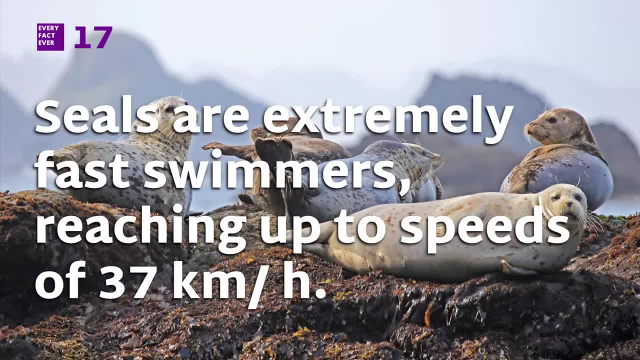 stay submerged for up to 30 minutes. Elephant seals can hold their breath for a remarkable 2 hours. Fact Number 17.. Seals are extremely fast swimmers, reaching speeds up to 37 kilometres per hour. Seals gain speed by porpoising or gliding on the water's surface to minimise resistance. 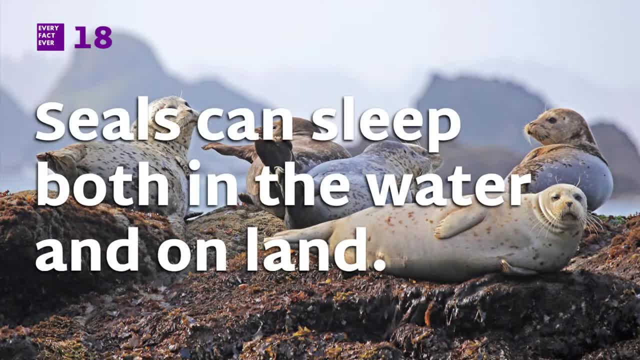 Fact Number 18.. Seals can sleep both in the water and on land. Seals sleep in water With half of their brain awake. however, when on land, both sides of their brain goes into sleep mode. Fact Number 19.. 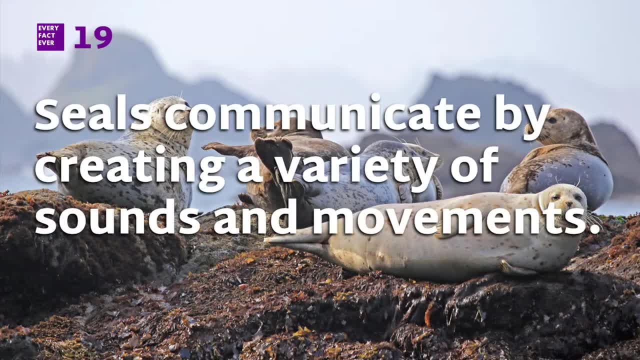 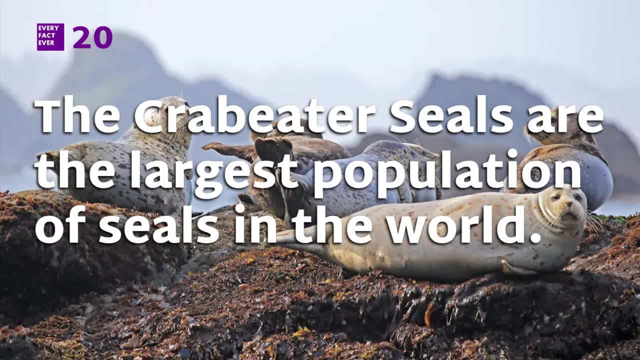 Seals communicate by creating a variety of sounds and movements. They can be heard making honking noises and even trumpeting sounds. Fact Number 20.. The Crab Eater Seals are the largest population of seals in the world. They are generally found in the Atlantic and their numbers range from 2 to 76 million. 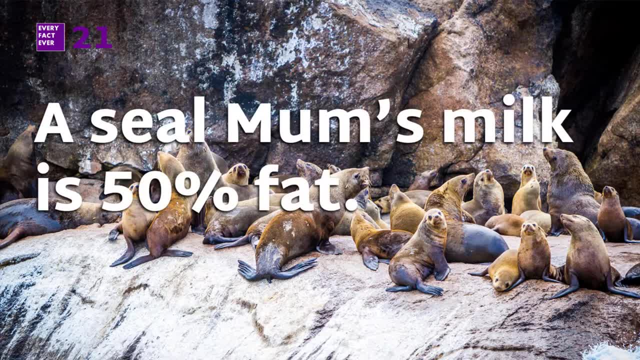 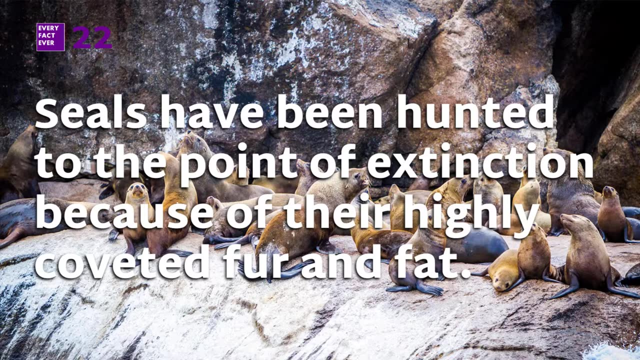 worldwide. Fact Number 21. A seal's mom's milk. Mom's milk is 50% fat. Researchers have observed that pups would gain 3 to 5 pounds a day because of their mother's milk. Fact Number 22.. Seals have been hunted to the point of extinction because of their highly coveted fur and fat. 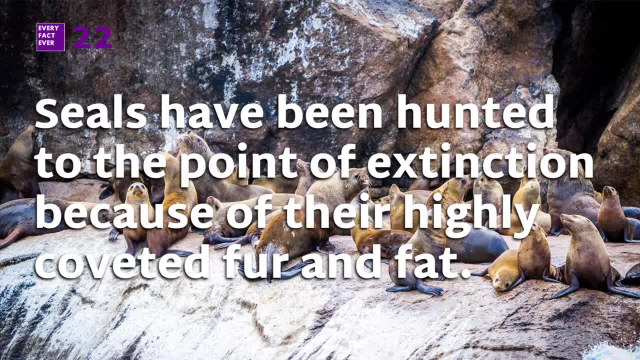 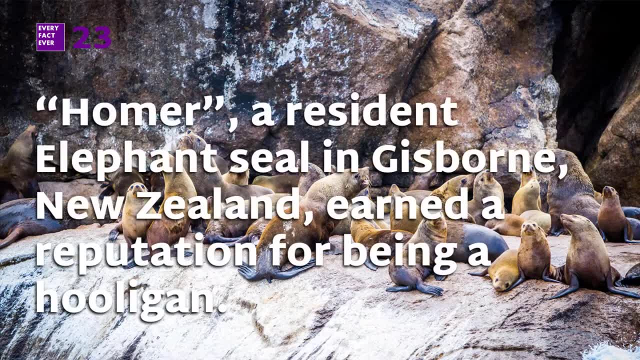 Coincidentally, the Galapagos fur seal is critically endangered and a highly protected marine mammal in most parts of the globe. Fact Number 23. Homer, a resident elephant seal in Gisborne, New Zealand, earned a reputation for being: 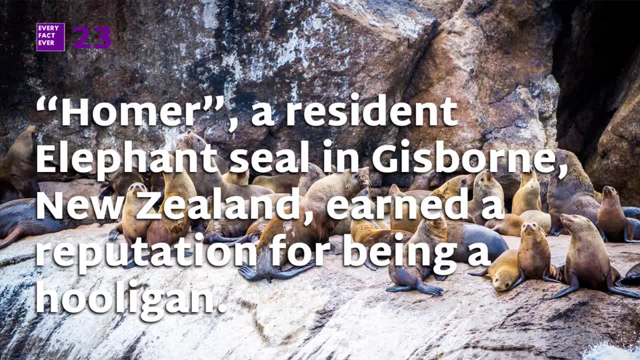 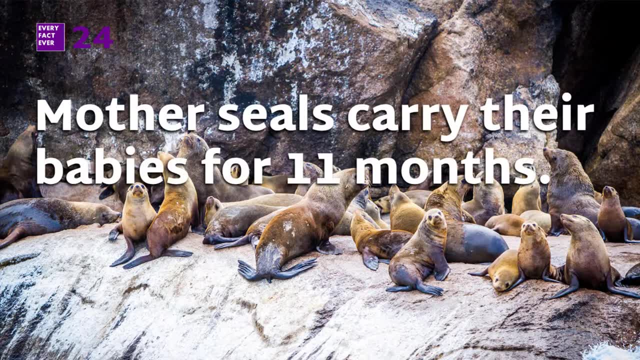 a hooligan. Her muse overturned parked cars and even knocked over a restaurant's power supply once. Fact Number 24.. Mother seals carry their babies for 11 months. The longest pregnancy in a pinniped family belongs to the walrus, with a 16-month gestation. 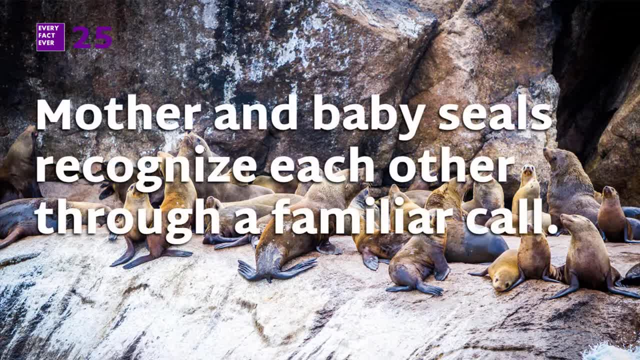 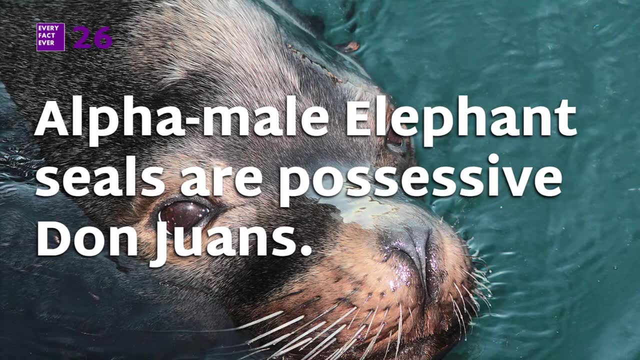 period. Fact Number 25.. Mothers and baby seals recognise each other through a family call. A study conducted in Alaska confirmed that the mom's pup's recognisation is even possible after a four-year-long separation. Fact Number 24.. Alpha male elephant seals are possessive donawans. 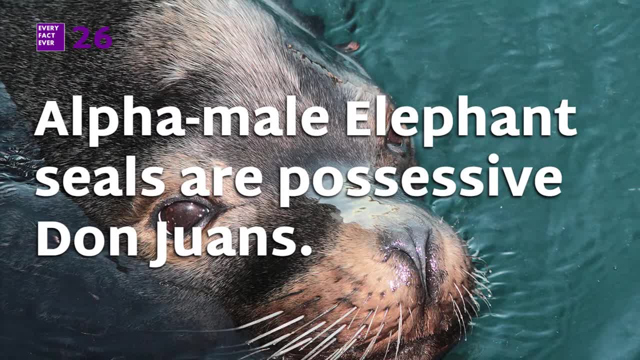 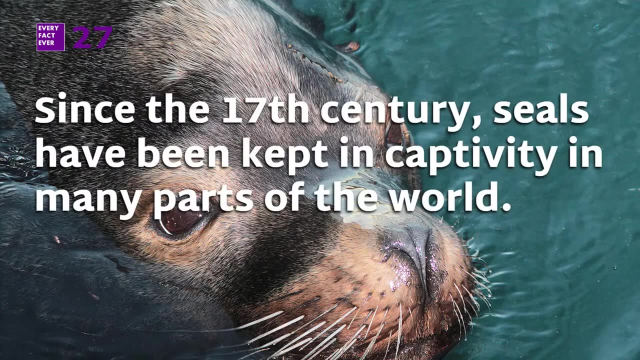 In one colony alone, more than 90% of the pups born are sired by a group of alpha males, and 72% of the male population in that colony may never experience mating at all. Fact Number 27.. Since the 17th century, seals have been kept in captivity in many parts of the world. 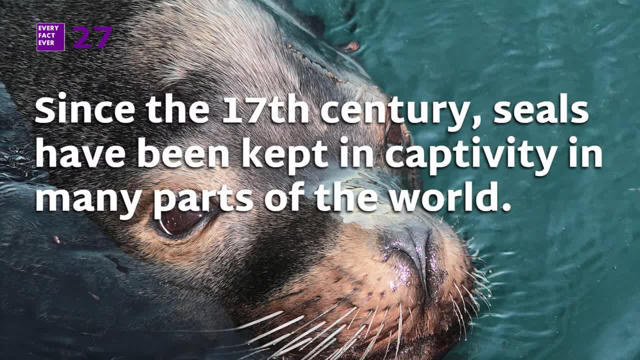 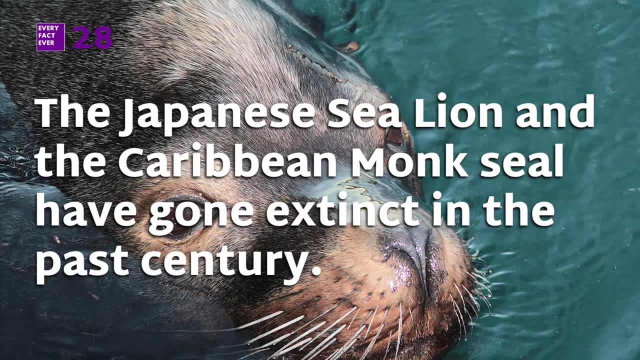 Captive seals make popular attractions at sea parks and zoos because of their large size and playfulness. Fact Number 28.. The Japanese sea lion and the Caribbean monk seal have gone extinct in the past century. The Mediterranean monk seal and the Hawaiian monk seal are listed as critically endangered. 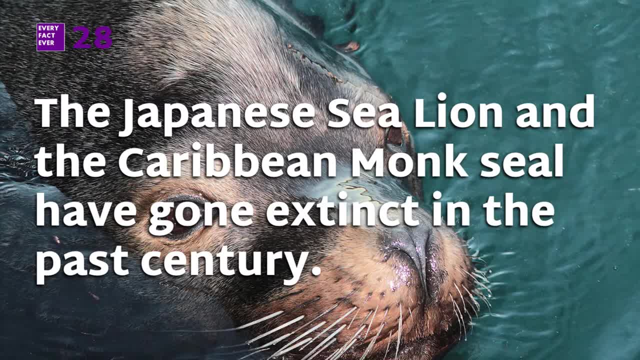 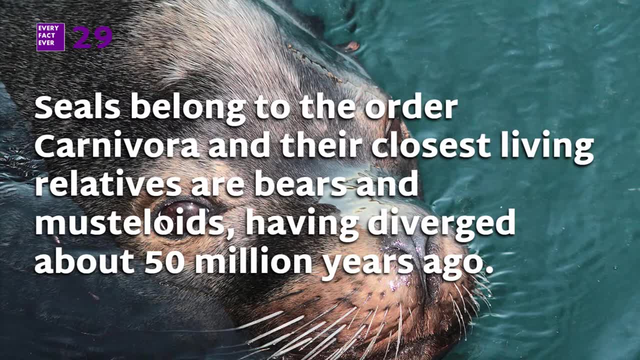 by the International Union for Conservation of Nature, Fact Number 29.. Seals belong to the order Carnivora and their closest living relatives are bears and musteloids, Having diverged about 50 million years ago. 50 extinct species of seals have been discovered. 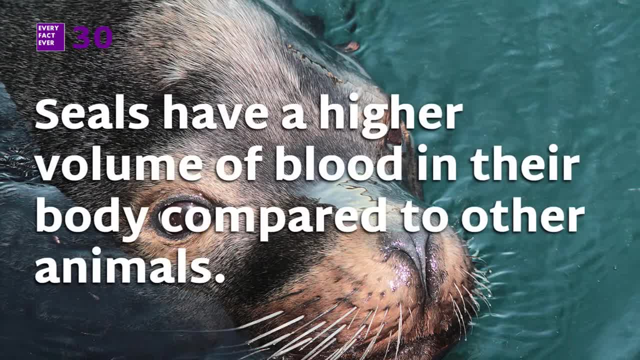 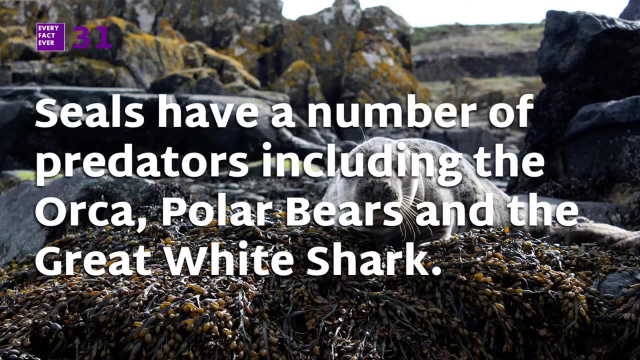 in fossils. Fact Number 30. Seals have a higher volume of blood in their body compared to other animals. Seals have an increased amount of myoglobin in their blood, which is the protein that stores oxygen. Fact Number 31. Seals have a number of predators, including the orca, polar bears and the great white. 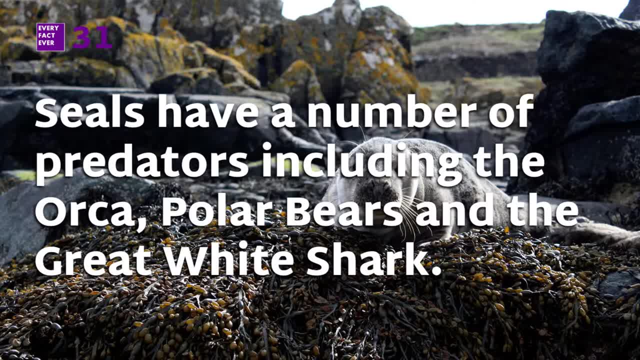 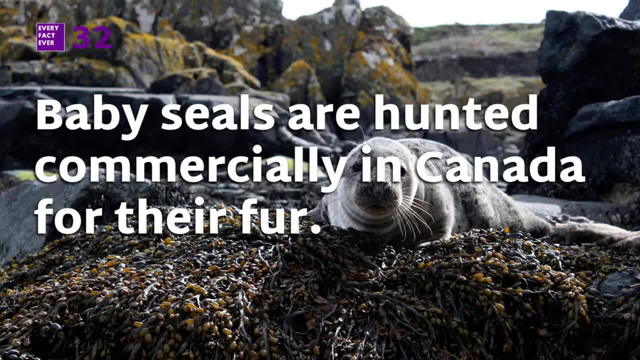 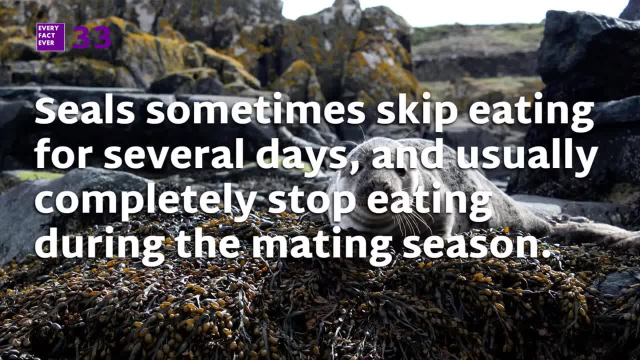 The seal's fur is highly coveted in the fashion industry. invasion against human beings- Fact Number 33. Seals sometimes skip eating for several days and usually completely stop eating during the mating season. During these times, they rely mainly on the energy stored in their blubber. 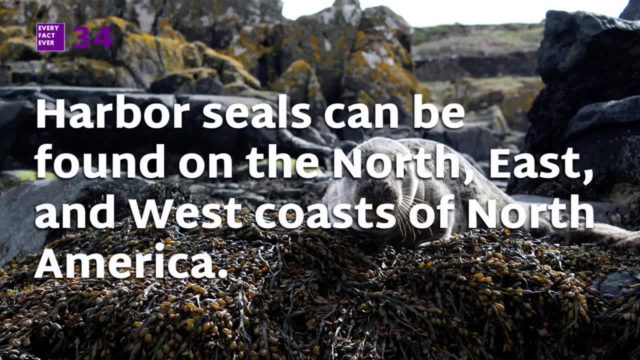 During these times, they rely mainly on the energy stored in their blubber. Baby seals live in warm أن 신받을 속을티는 안 norte. 외국어- fact number 34.. Harbour seals can be found on the north, east and west coast of North America. 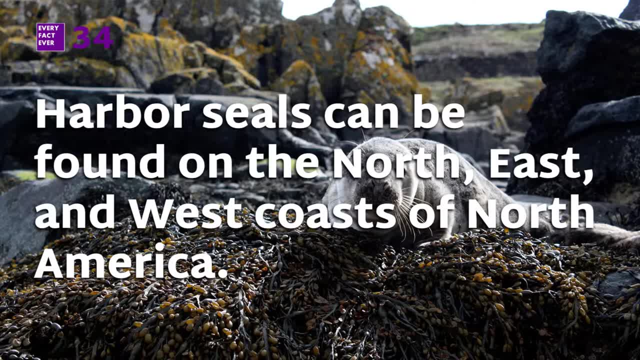 fact. In fact, you can find harbour seals in the Pacific Sea extending from northern Japan up to the Asian coast and across to Bristol Bay, Alaska, and down the coast to California. Fact Number 35. Males are not able to mate until they are 8 years old. 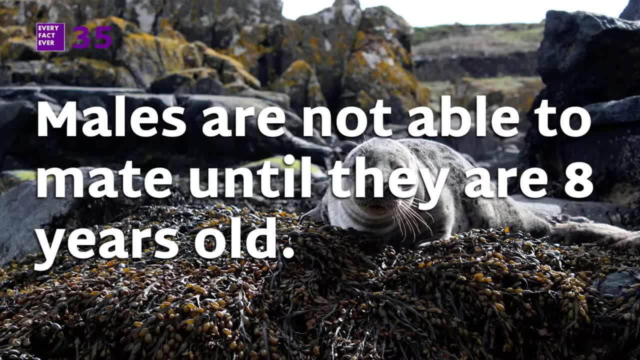 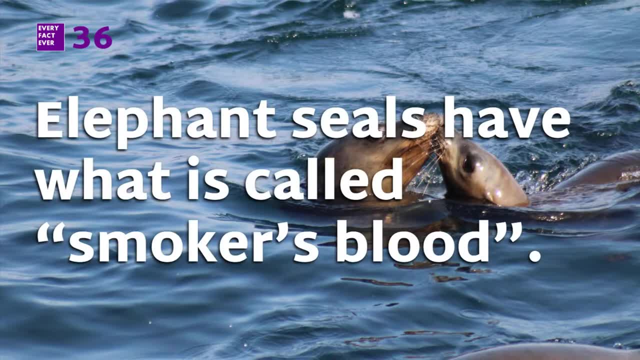 It takes male seals that long to grow big and strong enough to win a mating fight. Fact Number 36. Elephant seals have what's called smoker's blood. The amount of carbon monoxide present in the blood of an elephant seal is similar to a person who smokes 40 cigarettes a day. 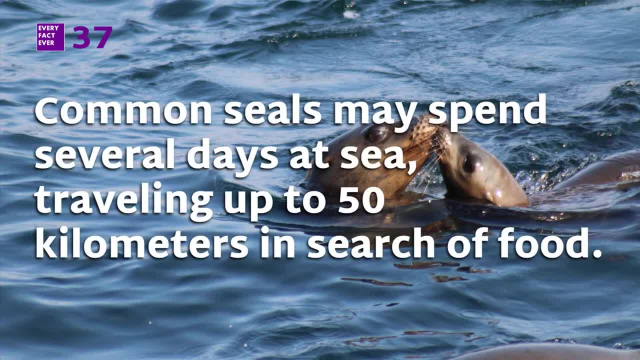 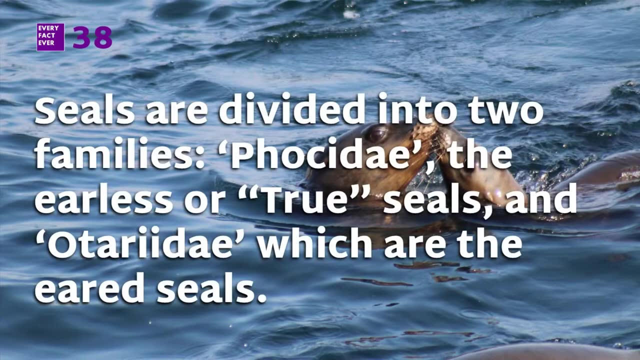 Fact Number 37. Common seals may spend several days at sea, travelling up to 50 kilometres in their search for food. They will also swim upstream into large rivers, resting on mudflats or on rocky coasts. Fact Number 38. Seals are divided into two families: Fossidae, the earless, or true seals. 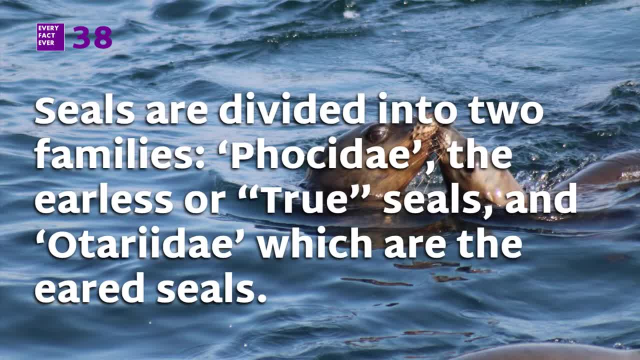 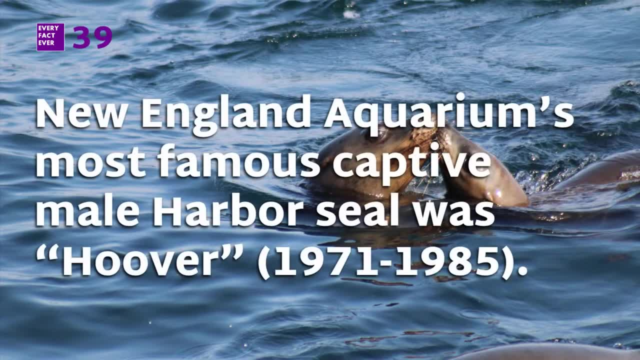 and Odoridae, which are the eared seals. True seals include harbour and common seals, whereas the eared seals include sea lions and fur seals. Fact Number 39.. New England's aquarium's most famous captive male harbour seal was Hoover. 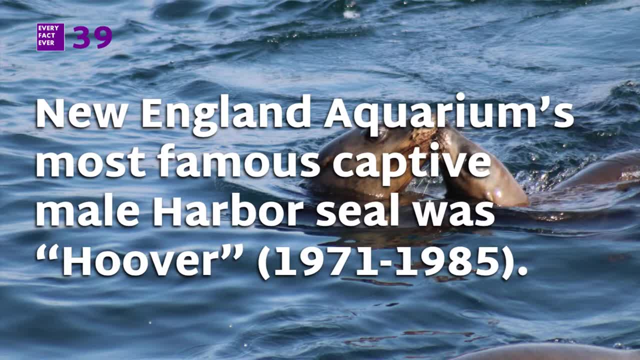 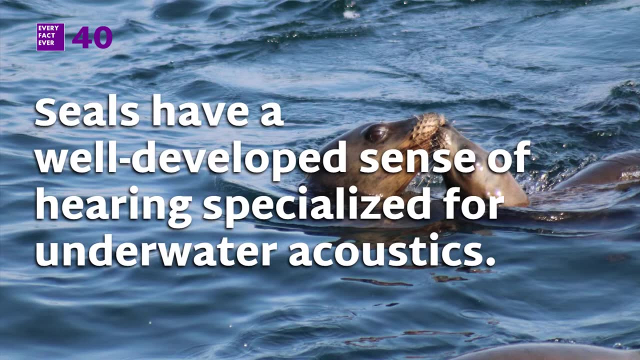 who lived from 1971 to 1985.. Hoover even managed to learn how to say hey, hey, come over here in a noticeable New England accent, among a few other phrases. Fact Number 40. Seals have a well-developed sense of hearing, specialised for underwater acoustics. 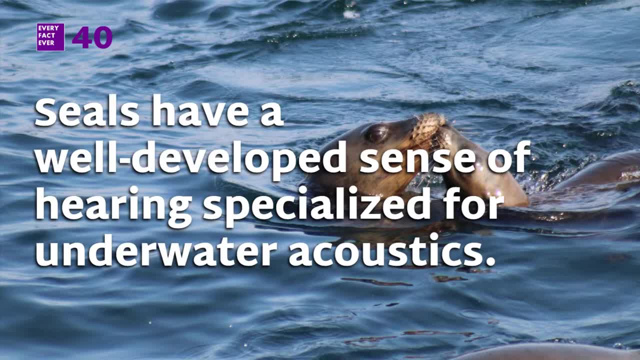 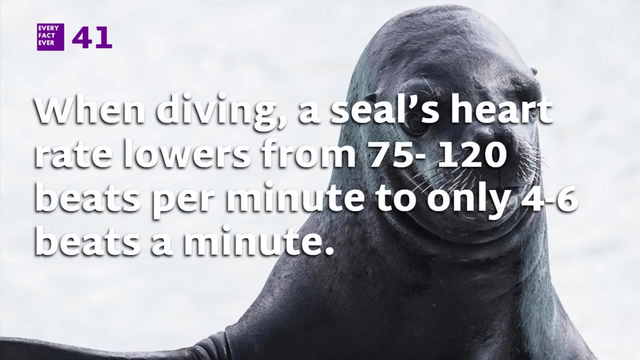 Seals are able to respond to sound from 1 to 180 kHz underwater. However, when at surface, their hearing ability is reduced to only 1 to 22.5 kHz. Fact Number 41. When diving, a seal's heart rate lowers from 75 to 120 beats per minute. 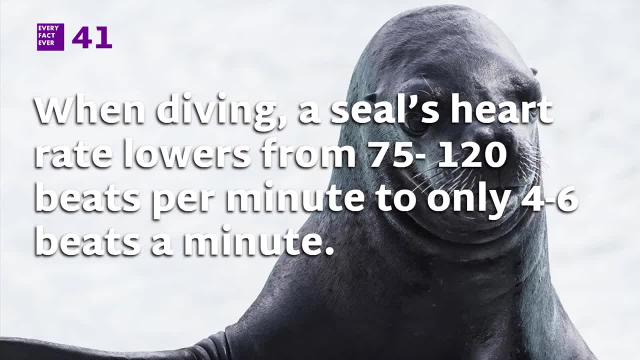 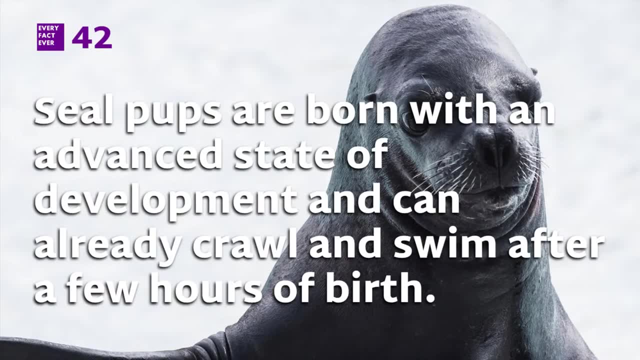 to only 4 to 6 beats per minute. Adult seals experience bridal cardio lowering of the heart rate at the start of each dive. Fact Number 42.. Seal pups are born with an advanced state of development and can already crawl and swim after just a few hours of birth. Pups are normally born on shore. 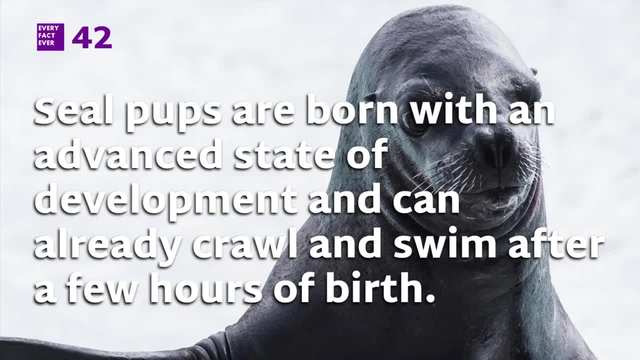 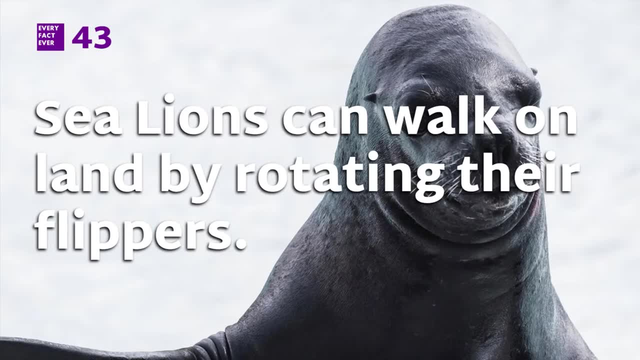 beginning in February for populations at lower latitudes and as late as July for those in the sub-Arctic regions. Fact Number 43.. Sea lions can walk on land by rotating their flippers. The same cannot be said for true seals. 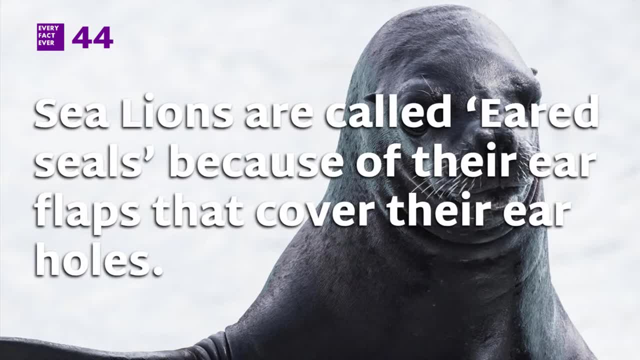 Fact Number 44.. Sea lions are called eared seals because of their ear flaps that cover their ear holes. Another contrasting characteristic among seals and sea lions is the presence of fur that covers the animal's long claws, which the seal's seal lines have, but true seals don't. 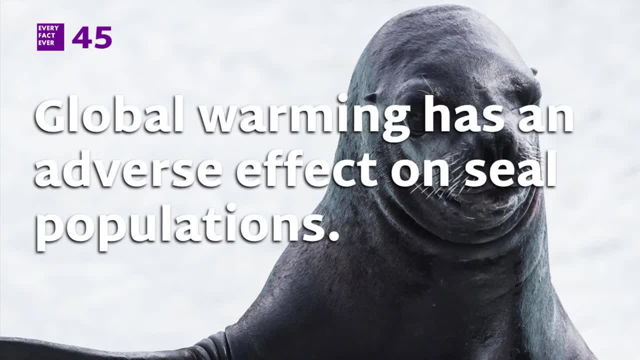 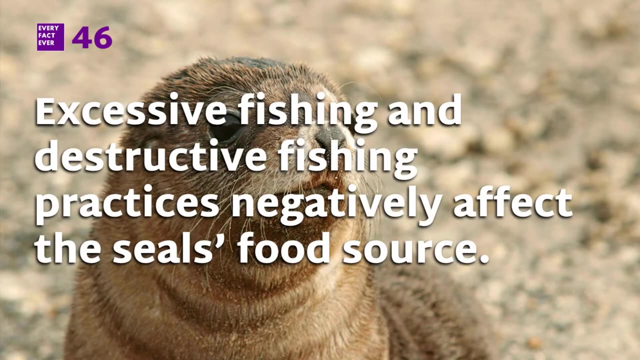 Fact Number 45.. Global warming has an adverse effect on seals' populations. As the Earth's surface warms up, the seal's excessive blubber, instead of protecting the animal from the cold, is starting to become a negative characteristic. Excessive fishing and destructive fishing practices negatively affect the seal's food source. 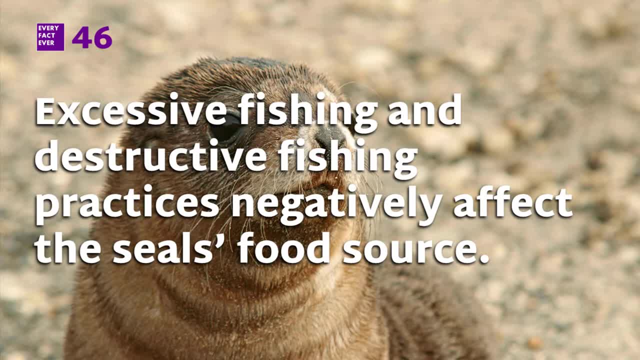 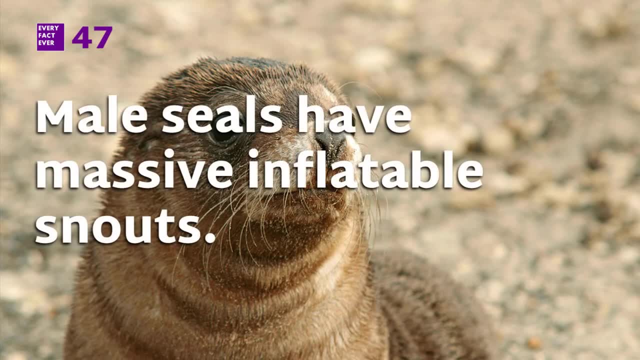 Seals may have to migrate for hundreds of miles to search for crab, krill and other staples of their diet. Fact Number 47.. Male seals have massive inflatable snouts. A male seal's most conspicuous feature is his bulbous nose that comes with a proboscis. 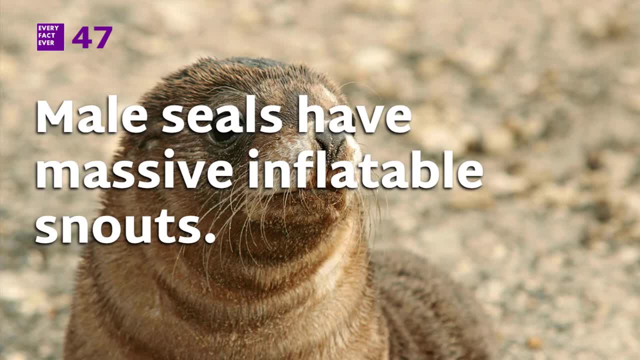 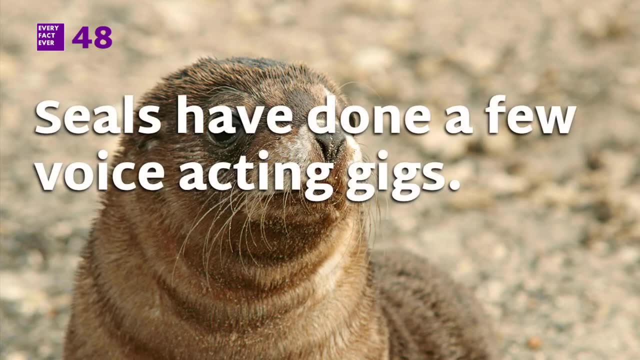 which is a sack-like appendage used to amplify grunts, snorts and the seal's loud drum-like bellow. Fact Number 48.. Seals have done a few voice acting gigs. The cries the elephant seal pups make were the inspiration for producing the cave-dwelling Moria. 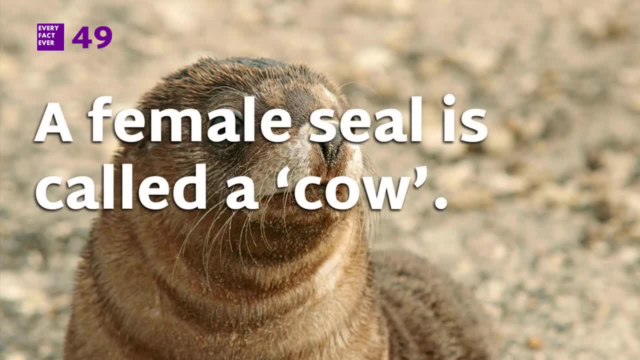 orc's eerie battle screech. Fact Number 49.. A female seal is called a cow. A female seal or cow gives birth to only one pup once a year on land and nurses the pup for about four days to a month. 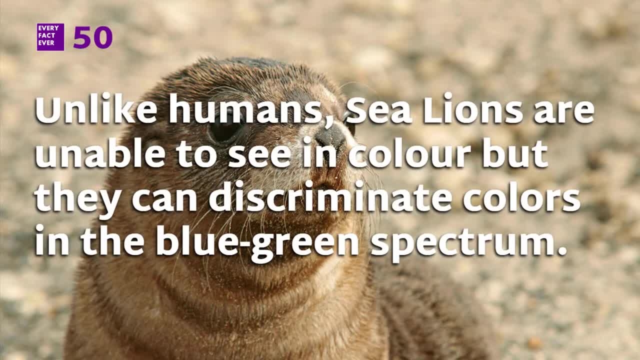 Fact Number 50.. Unlike humans, sea lions are unable to see in colour, but they can discriminate colours between the blue-green spectrum. Interestingly, like cats, all pinnipeds have a membrane at the back of each eye called tapidum.